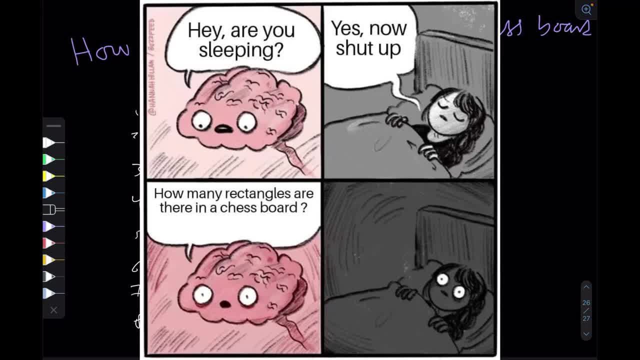 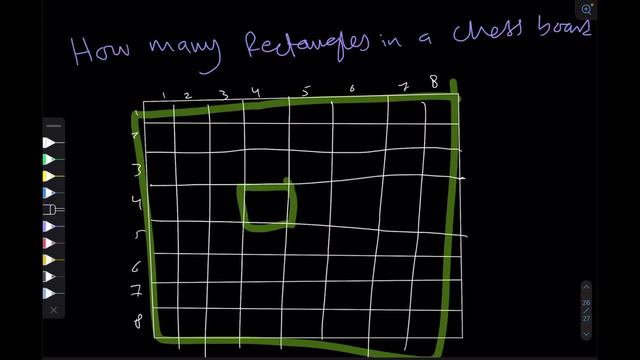 How many rectangles are there in a chessboard? So this whole square is itself a rectangle. Any small square is a rectangle, and of course, anything like this is a rectangle, And so we are trying to find out how many different, unique rectangles will there be. 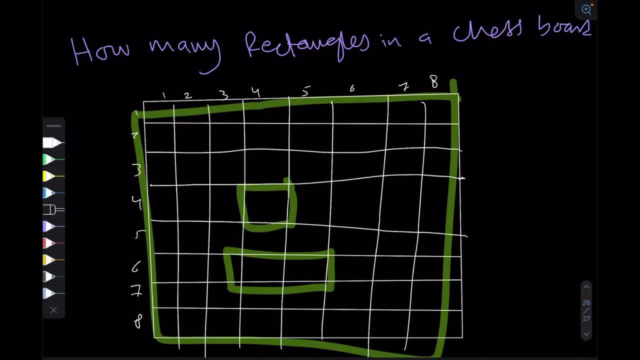 So when you start off with this problem, a major problem is that a chessboard is an 8x8 board and that's pretty big, So working with it could be a little hard. So what we can do is we can start with smaller numbers and we 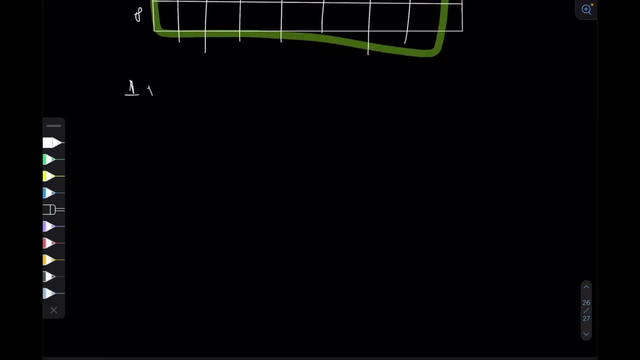 can look for patterns. So if we have a 1x1 square, there's just one rectangle. That's the only square Let's look at if we have 2x2's. So this thing, Well, there are, if you look at. 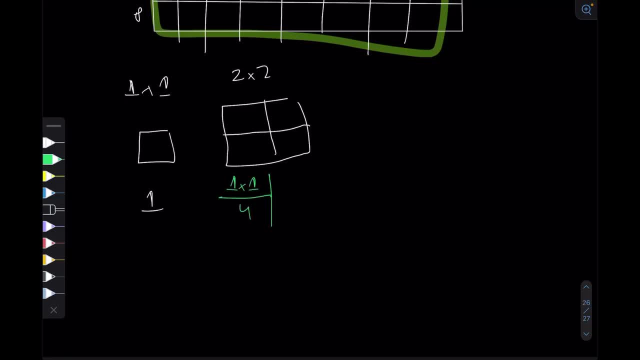 how many 1x1's there are. there are 4 of those, And then we can look how many 2x1's there are. There will be 2 of those. Similarly, if we look at 1x2's, there will be 2 of those And of course there will be 1 2x2.. 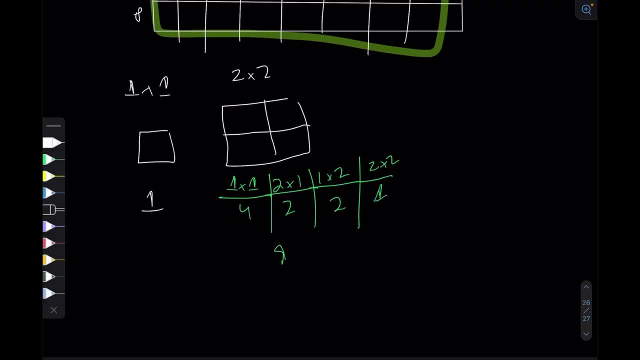 This would be equal to 9.. Let us also look at 3x3's now. So of course there will be 3 1x1's And then we can look at 2x1's. So like this, Like this, And then thrice of those. So 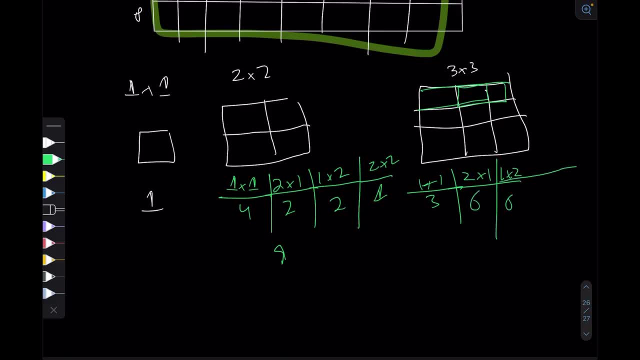 6. And similarly, 1x2's will also be 6. If we look at 2x2's- that is, a square like this- It will be 4 of those, And then we can look at 2x3's. 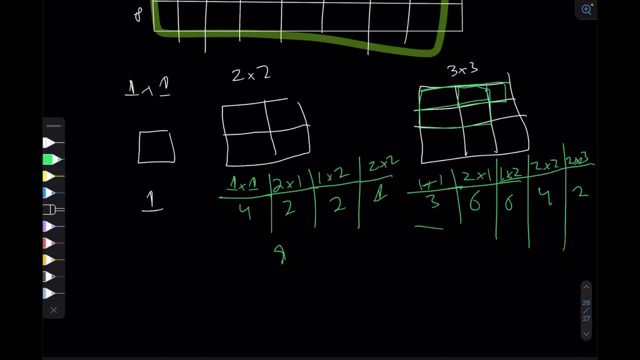 2x3's would be 2 of those, And of course 3x2's will also be 2.. And then 3x3 will be 1.. Sorry, there will be 9 1x1's. Oh, and I forgot 1x3's and. 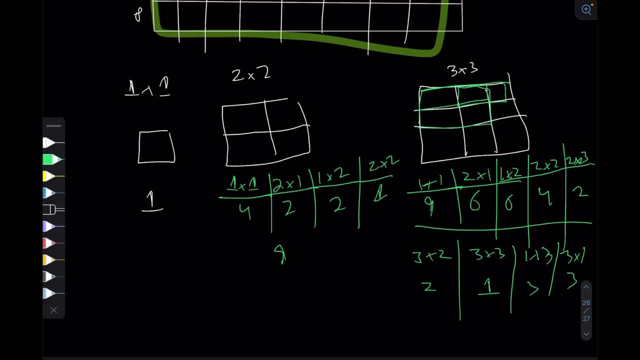 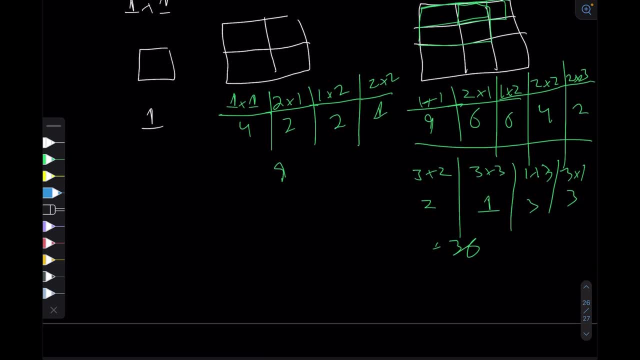 3x1's: 3 of those, 3 of those. This will turn out to be 36.. You can go over to 4x4's, but if we look at the current patterns that we have, As in, n equals 1, 2. 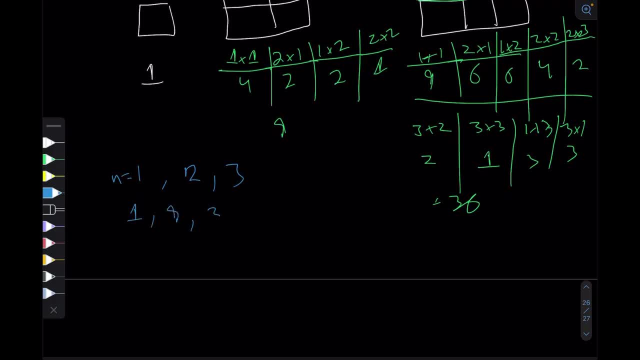 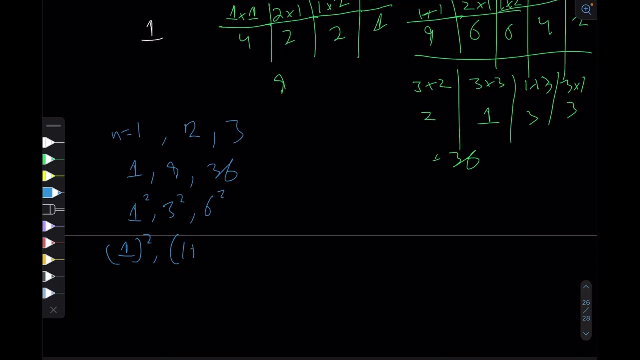 and 3.. We have 1, 9 and 36.. We can notice that these are actually 1 squared, 3 squared and 6 squared, And so we can see that this would be like 1 squared and then 1 plus 2 squared And then 1 plus. 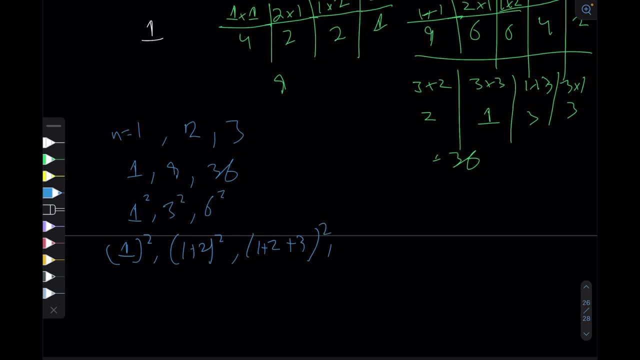 3. Sorry, 1 plus 2 plus 3 squared, And so on. Another thing that we might reduce from this is that if we want to go from n equals 1 to 2. We are adding 8, from 2 to 3. We are adding 27.. 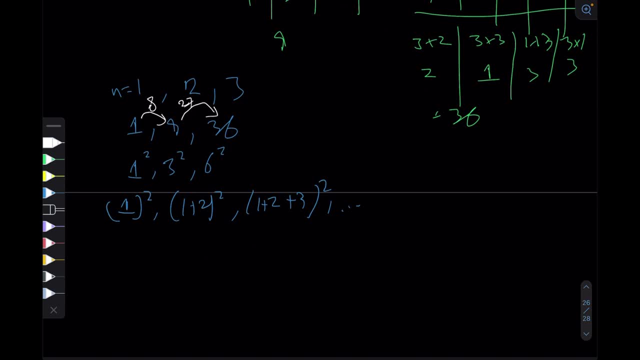 So this could basically be 1 cubed, 1 cubed plus 2 cubed, 1 cubed plus 2 cubed plus 3 cubed, and so on, And actually both of these are really the same because the sum of natural numbers from r equals. 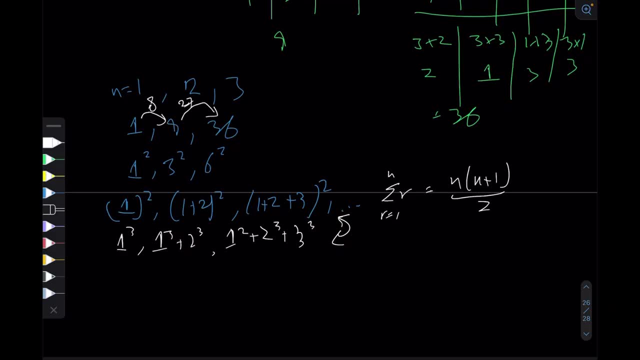 1 to n is basically n? n plus 1 over 2. And if you want to square them, it would be this: And the sum of the cubes is also actually the same formula. that is easy to prove by induction. So we can go ahead and try to prove this. So we can. 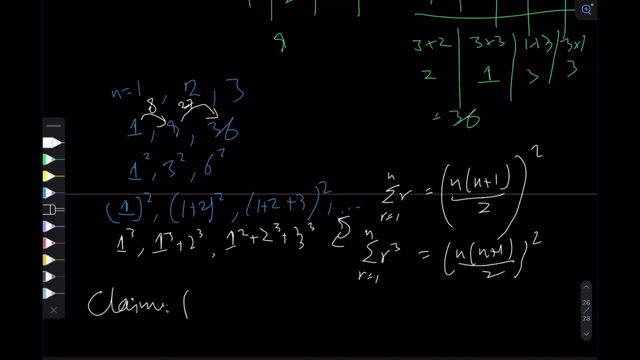 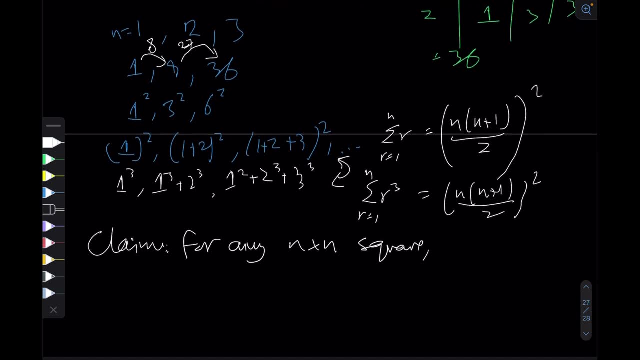 claim that for any n by n squared total number of rectangles is the same as the sum of natural numbers from 1 to n, and then you square it. In other words, it would be n? n plus 1 over 2 n squared Right. So. 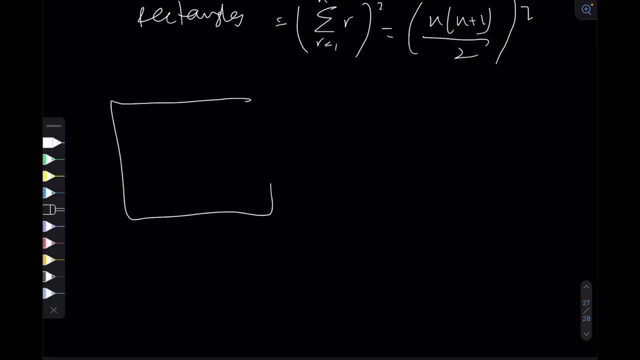 we can. What we can do is: So let's say, there is a 3 by 3.. Right, And we can basically track how many 1, 2 3's and 1 2 3's there are, and hopefully we can see some sort of a pattern. 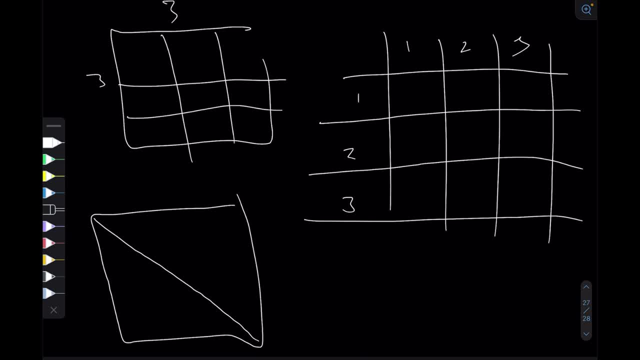 So one thing to notice would be that this chart would be actually symmetrical, as in: whatever is the stuff over here would be the stuff over here too, because since it's a square, the total number of m by n's is the same as the total number of n by n's. 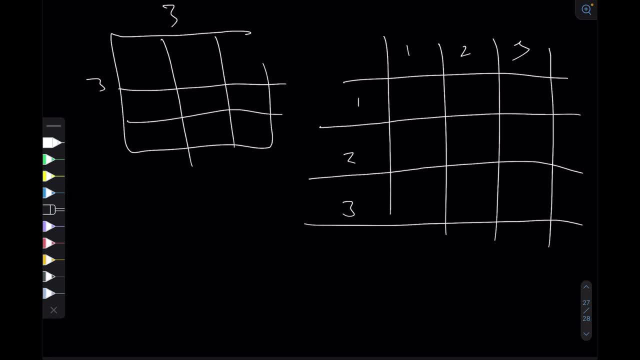 Right, So let's do the easy ones first. 1 by 1, there is, of course, 9 of those. If you look at 3 by 3, there is just 1 of those. 3 by 2 would be 2 of those, and 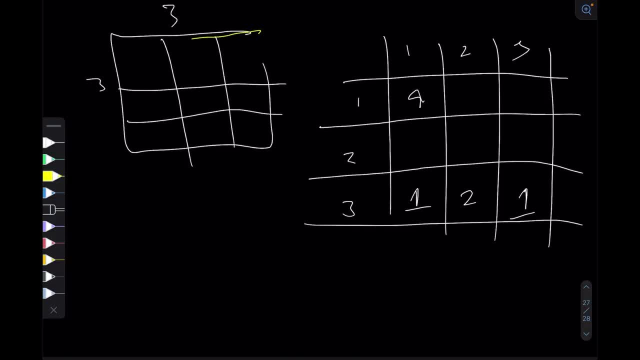 3 by 1 would be 1 of those Right, Simply because this is your whole 3 by 3.. So if you have 3 by 2's, you can split it up like this and then like this, And then if it's 3 by 1, you can further. 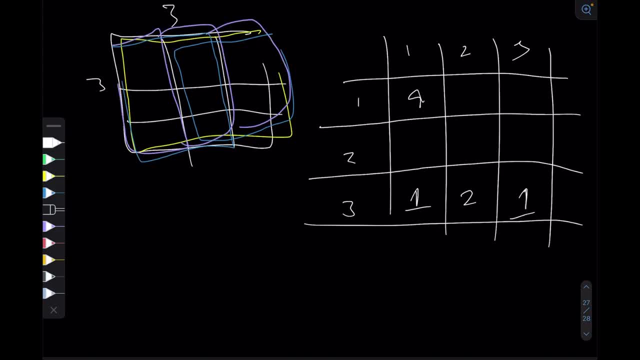 split it up like this Right. So from this sort of procedure we can see that if we have a 3 by 3, if we have n numbers of 3 by 3, then there will be twice number of 3 by 2.. So if we have 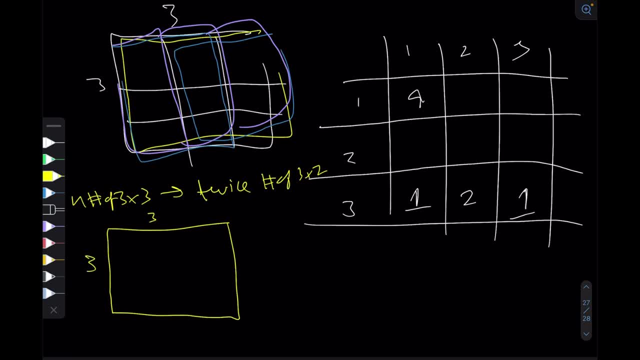 a 3 by 3. let's say this is 3 by 3. every 3 by 3 can be split up into 2- 3 by 2's. This would be one of them, and then this would be another one of them. 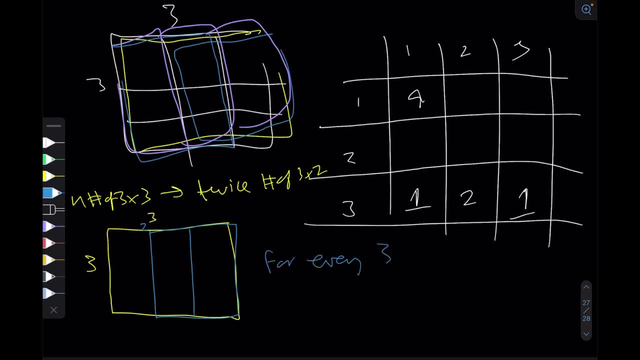 So for every 3 by 3, there are twice 3 by 2's, So there are 2. sorry, yeah, there is 2 of 3 by 2's. And so, by very similar logic, we can notice a similar algorithm that if there are. 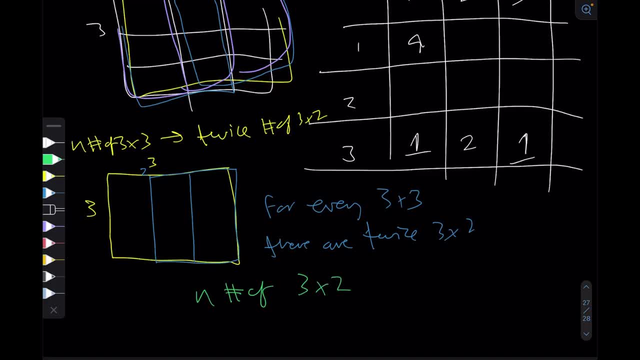 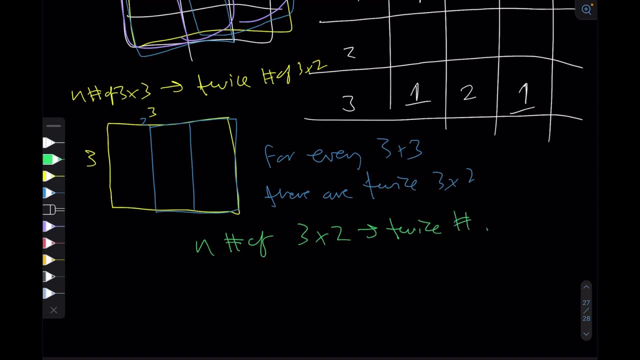 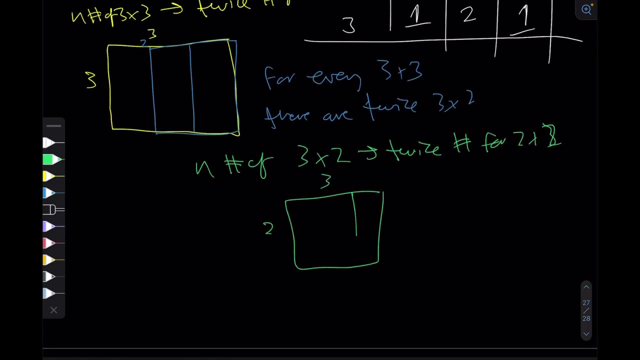 n number of 3 by 2's, there will be twice the number for 2 by 2's- 2 by 2's, because every 3 by 2 can be split up into 2 of 2 by 2's One. that will be this. 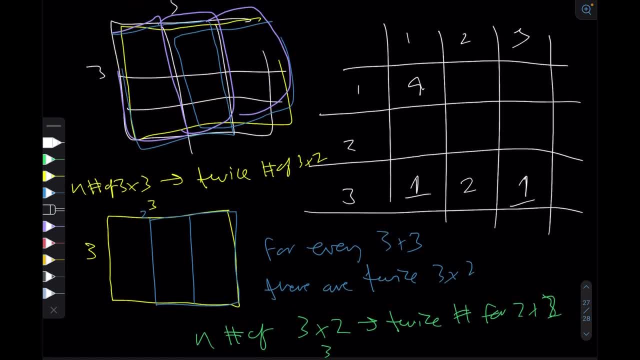 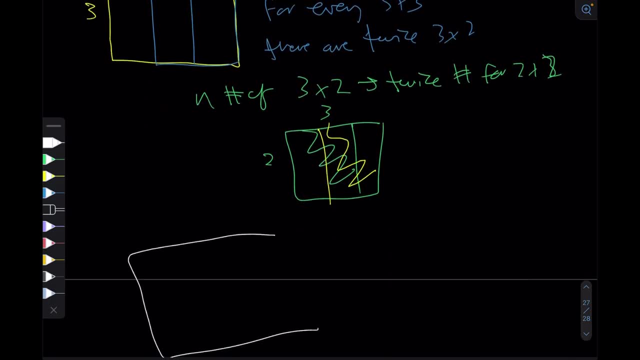 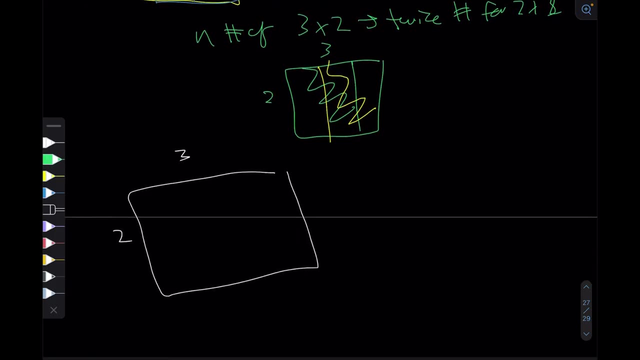 and another one. that will be this. So we can continue on and say that this will be 4 and then this will be 6, because if we have any, if we have any 3 by 2's, then we can split this up into 3 of 2 by 1's. 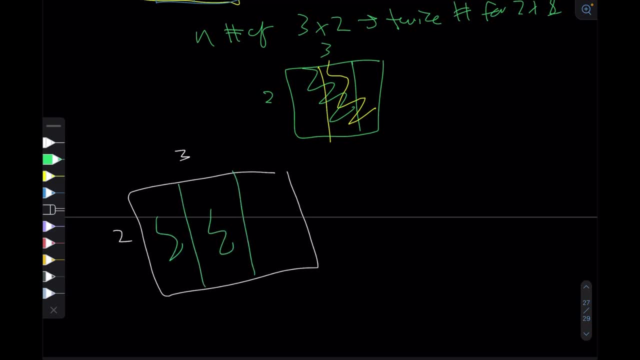 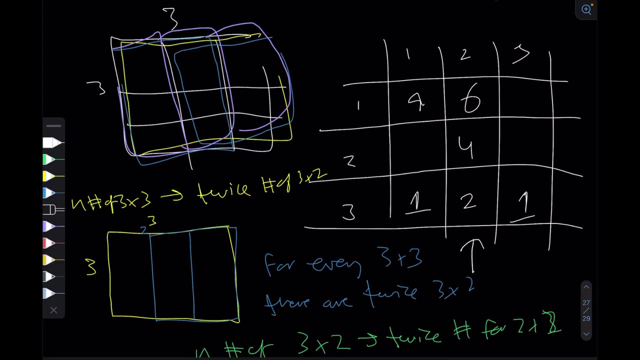 one like this. one like this: here is your 1, 2, 3, so we can see that this would basically be the multiples of 2, 2, 4, 6, 8, all the way right, and when you continue on the same algorithm to 1 by 3's. 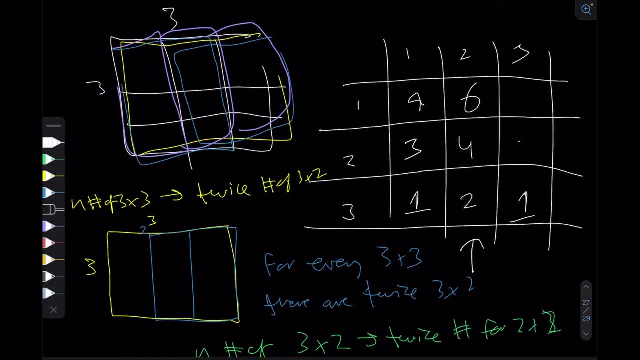 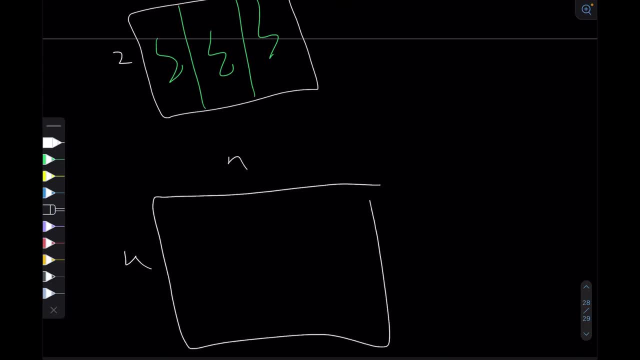 it would be 3, and this would be 1, 2, 1, 2, 3, right, and so what we can see is, for any n by n, here is your 1, 2, 3, all the way to n, 2, 3, wait. 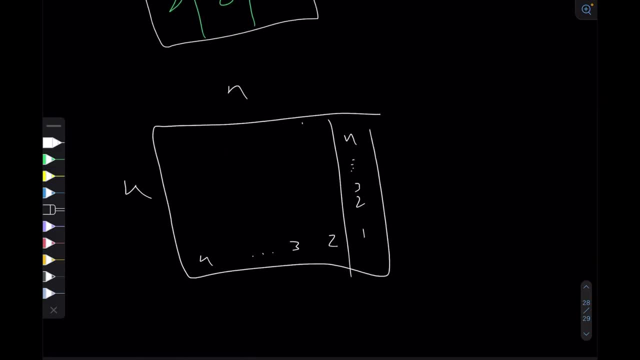 yeah, 2, 3 all the way to n, and then this would be the multiples of 2, that is, 2 times 2, 2 times 3 all the way to 2 times n. this would be the same for 3, and then this would be: 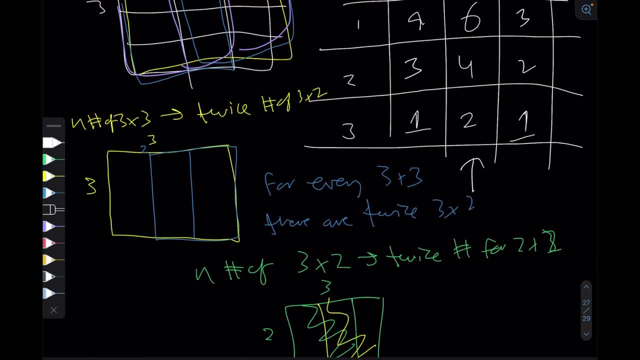 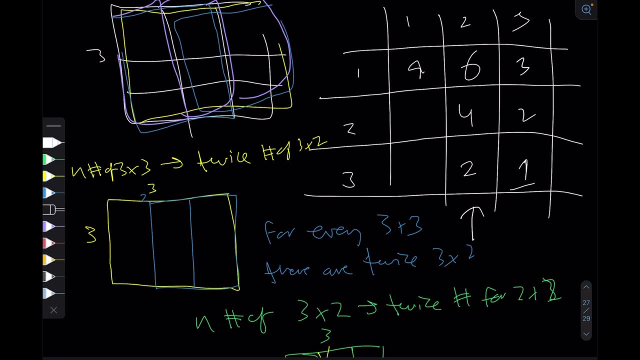 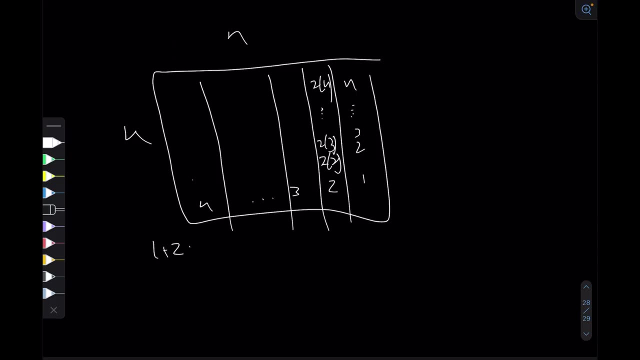 the same for n and so on. wait, this should be 3 of those, sorry, this should be 3. and then 3 times 2 is 6, and so on. so what we can see is that we have 1 plus 2 plus 3, all the way to n. 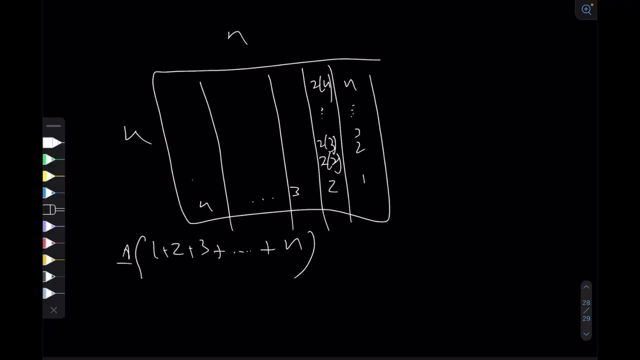 and then just this, and then you do the same thing, but you multiply it by 2, and then you do the same thing, you multiply it by 3, and you continue this all the way till you have n, and you are multiplying it with the same number. 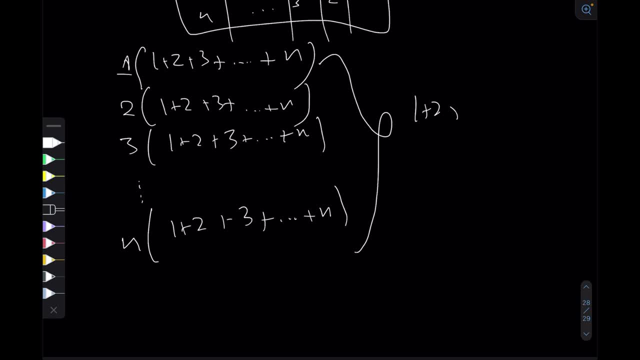 right, so we can group these into 1 plus 2 plus 3 all the way to n, and then you multiply it with 1 plus 2 plus 3 plus all the way to n. in other words, we have proved that this would be equal to 1 plus 2 plus. 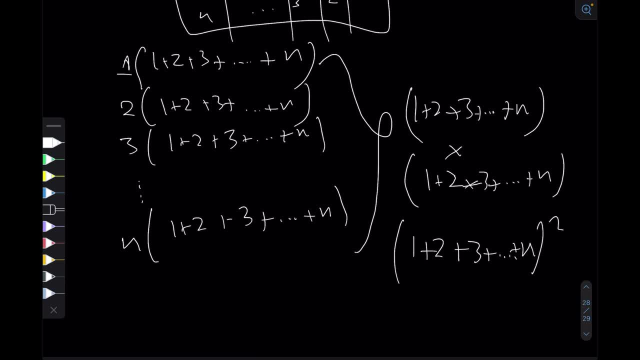 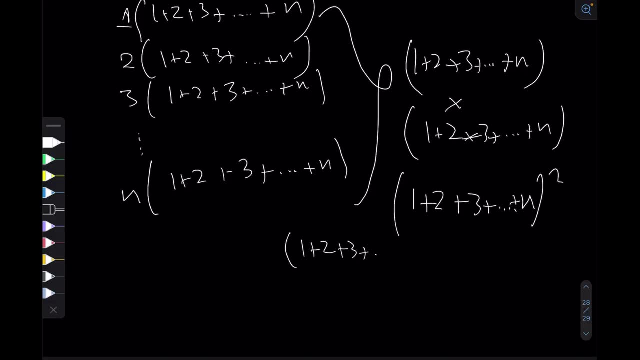 3 all the way to n squared. and so, if you want to answer the initial question of chessboard, that would basically be equal to 1 plus 2 plus 3 plus all the way to 8 squared. which turns out to be. it turns out to be. 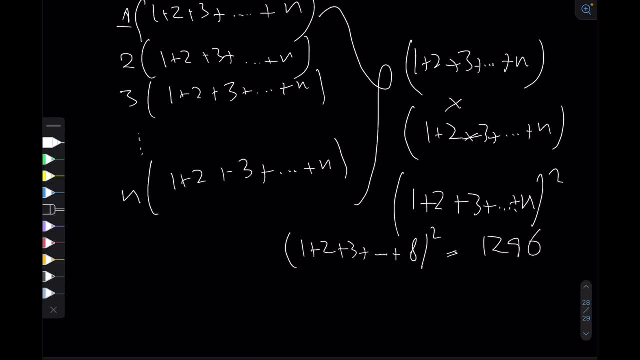 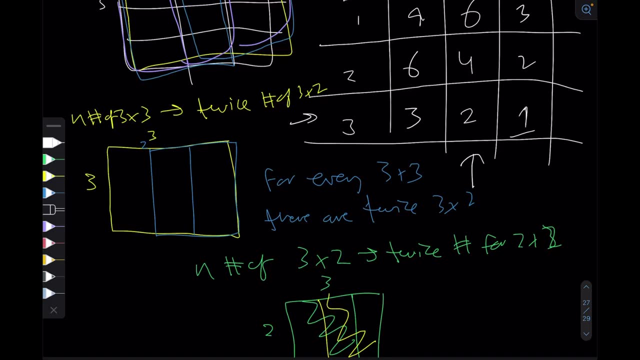 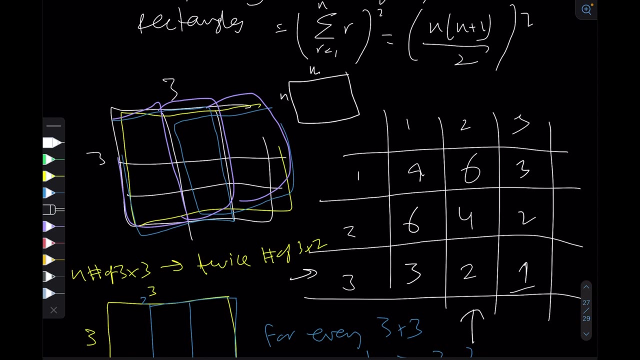 1296 and we have our answer. so above I sort of you know, took just one example and then I didn't generalize it, although I should have that. you know, if you have any m by n and then you are looking at m by n minus 1, you have to. 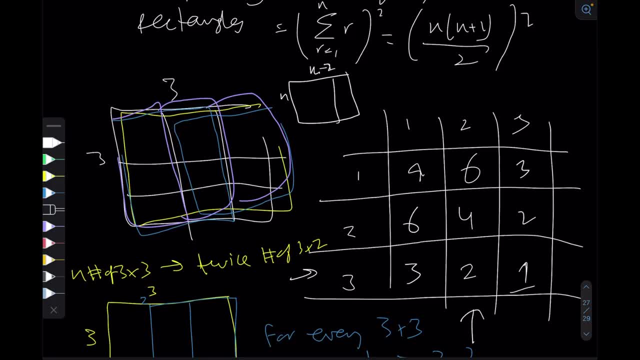 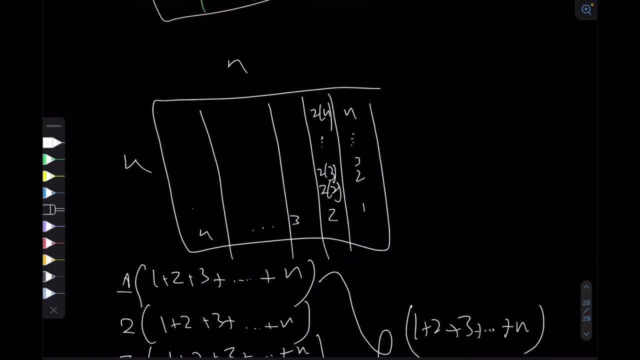 have twice of those for m by m minus 2, you will have thrice of those, and so on. but you know, you get the point and so we have reached at our answer. but there is one very much cooler way of doing this and it is by a combinatorics.